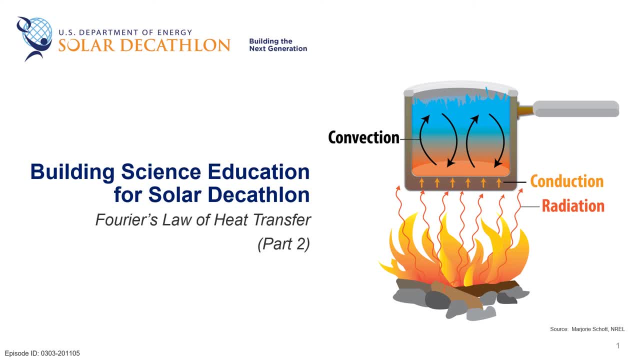 Welcome to the Solar Decathlon Building Science Education Series. I'm Paul Torsolini, and this episode is part two of our discussion of Fourier's Law of Heat Transfer. If you haven't watched part one yet, I recommend starting there to learn more about the fundamentals of how heat flows. 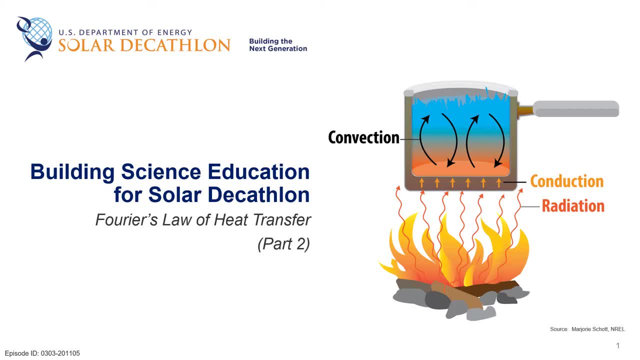 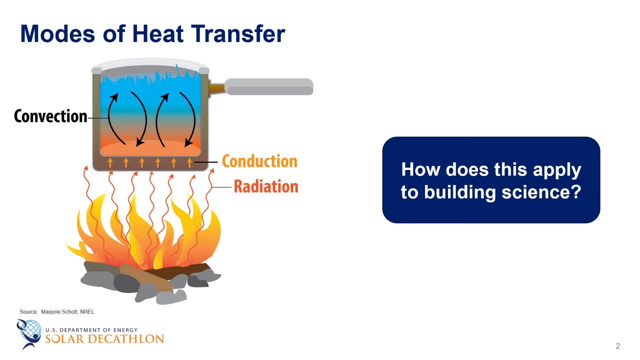 But if you have watched part one already, then let's get started with part two. In part one of our Fourier's Law episode, we defined these three distinct modes of heat transfer: conduction, convection and radiation. We used this illustration of a pot over a fire to help describe these processes. but now we want to talk about how this applies to building science. 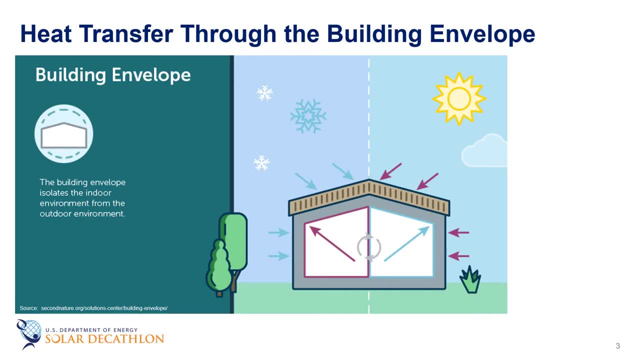 However, as with any thermodynamic problem, remember that we need to first define a boundary, and we're going to use that boundary to identify the temperature. We want to identify where heat transfer is occurring, And so, in a building, we call the portion of the structure that separates the inside comfortable temperature from the outside conditions the building envelope. 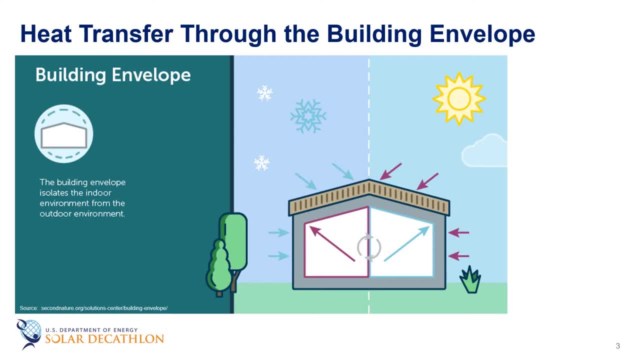 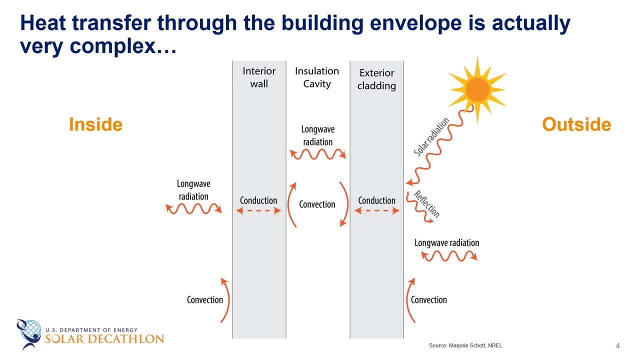 The exterior walls, the roof and the foundation floor all make up this thermal envelope, And examples of heat transfer exist at every component of the building envelope. As we look inside a wall, the first thing to note is that in many building science applications, 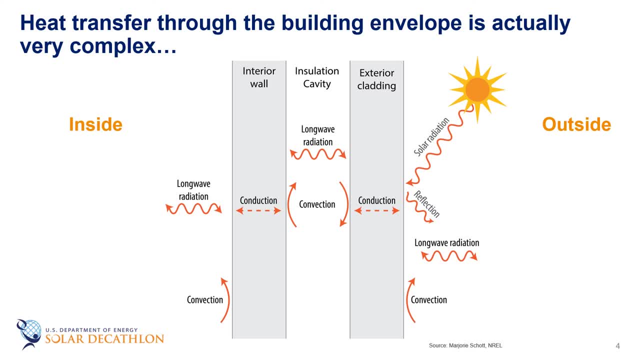 the transfer of heat is very complex, Often using two or three of the heat transfer modes at the same time. In the illustration here we see an exterior wall being made up of two solid components: the inner wall and the exterior cladding. And for the first example let's think of not having any insulation in the wall, so there's an air cavity between the two solid layers. 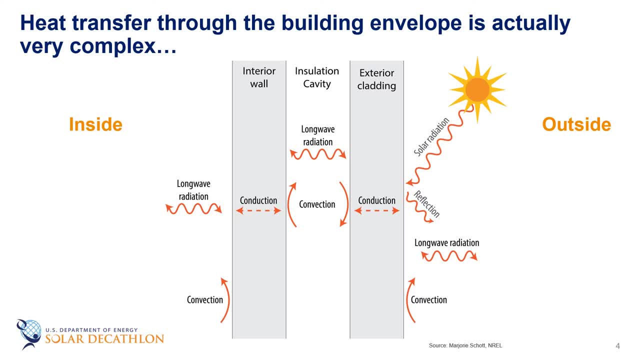 For the purpose of describing this illustration, we'll label the different surfaces, where location A is the inner surface of the inner wall facing the conditioned interior space of the building. Location B is the outer surface of the inner wall. Location C is the inner surface of the exterior cladding. 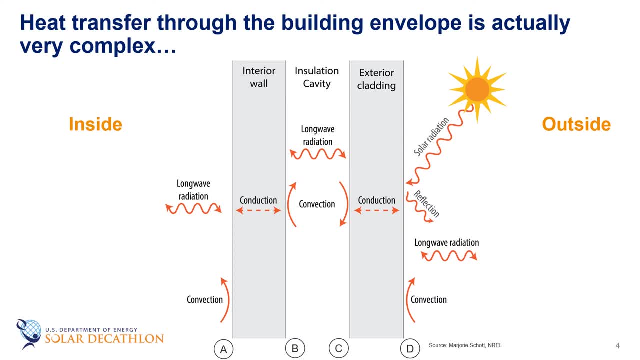 And location D is the outermost surface. As we look at the heat transfer through this wall, we'll see it occurring through all three modes. The first is radiation, Perhaps from the sun hitting the outside surface, Location D. There also appears to be convection in the outside air that's moving across the surface of the wall. 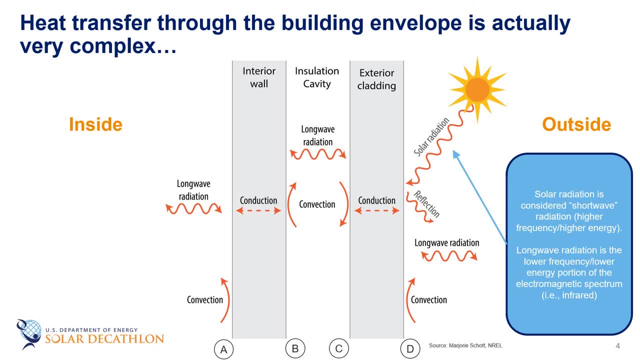 The wall itself may be solid and therefore it has conduction, But then we get to the air cavity. There is a temperature difference between location B and location C. This creates convection in the air cavity as well as long wave radiation. Moving then to location A inside the room. 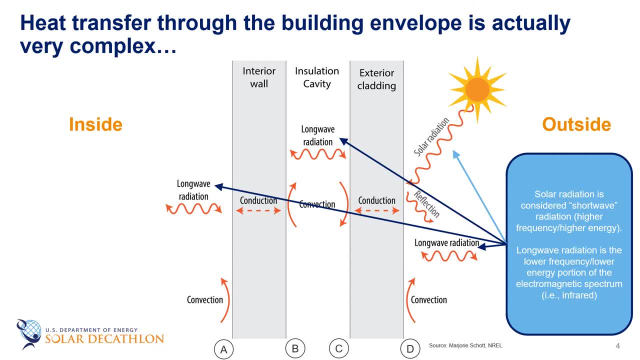 The wall is probably a little bit cooler than the room, So it's going to set up convection coefficients as well as long wave radiation to the space. At the end of the day, we need to take all of this complexity and we need to think about it as a model. 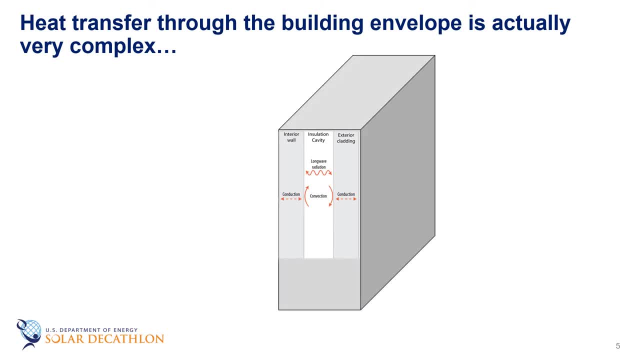 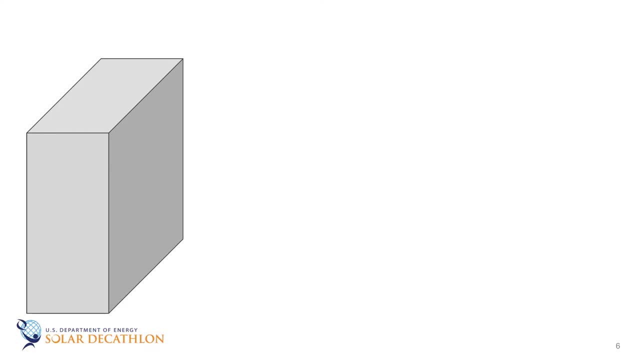 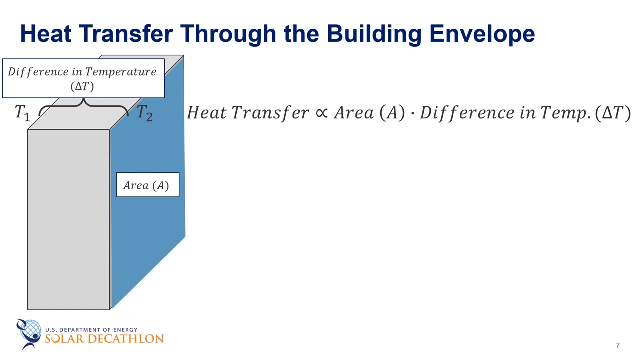 And we're going to simplify this so that it all approximates something that looks like conduction. With those assumptions, we can say that heat transfer is proportional to the cross-sectional area of the wall times the temperature difference. It's important to note that we said these are proportional to each other and not equal. 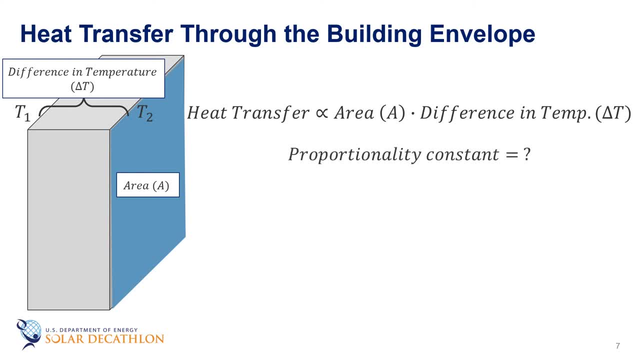 For these terms to be equal, there's something called a proportionality constant that needs to be factored in. We'll get to that in a moment, But first let's explain these other terms. Let's take a simplified section of a wall. 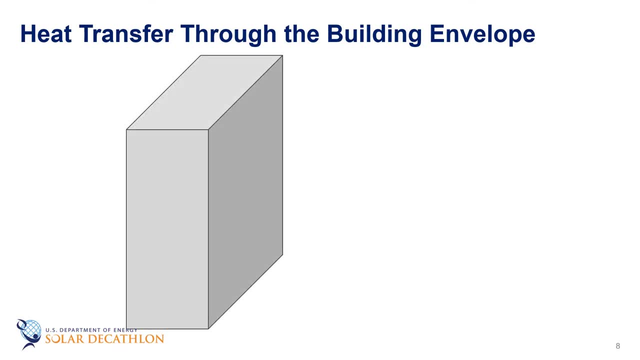 And remember that we're modeling this as conduction through a solid wall, But in reality there is also a small amount of convection and radiation occurring, And so we'll say we're in the middle of wintertime And so it's warm inside the house and it's cold outside. 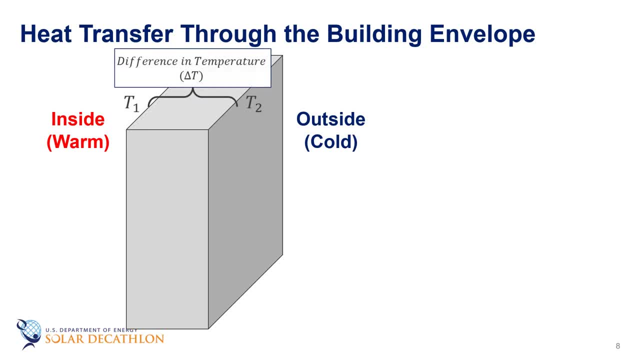 Because it is warm on one side and cold on the other side. there is a temperature difference, or a delta T, which drives the heat transfer. In this case, heat will flow through the wall from the inside to the outside And the rate of heat transfer will increase as this temperature difference increases. 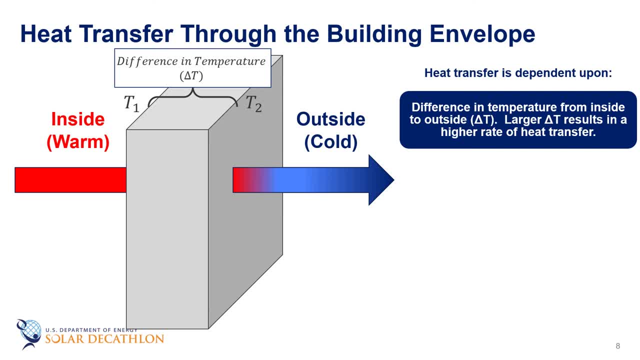 meaning, as it gets colder outside, heat is going to want to flow through the wall faster. The next thing that heat transfer depends on is the cross-sectional area of the wall. Let's call this A for area. The larger the area, the more heat transfer. 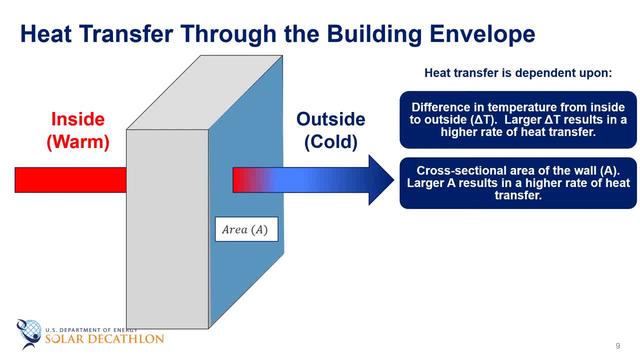 Think of the surface area of the wall as perhaps how much paint you have to apply to the exterior wall. Now what about the wall itself? The rate of heat transfer depends on what the wall is made of and how resistant those materials are to heat transfer. 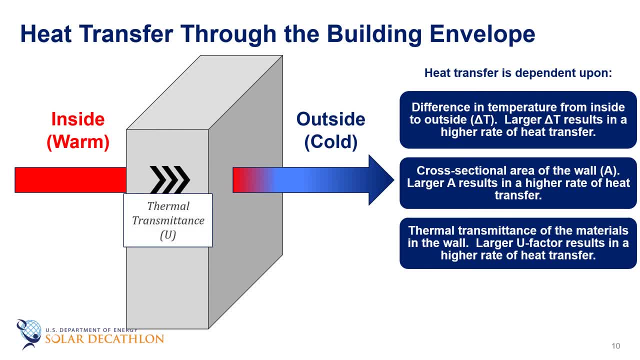 Notice where the proportionality constant comes in. We'll call this the U factor, And it is the coefficient of heat transfer of a material, in our case the wall. Put simply, the U factor represents the wall's thermal transmittance. 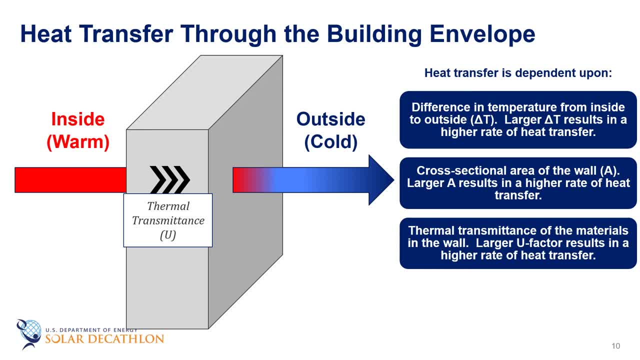 Higher U factors mean a higher rate of heat transfer. For a homogeneous material, the U factor is equal to the thermal conductivity of the material divided by its thickness. Walls typically consist of many layers of materials, so the derivation of the U factor for a wall is much more complicated. 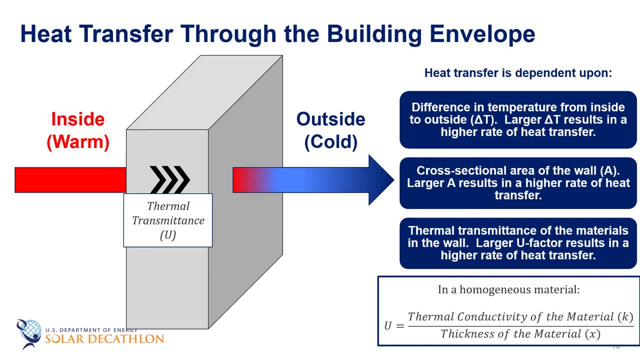 We'll cover that a little bit more later in the course. Thermal conductivity is a characteristic property of different materials. Some materials are highly conductive, while others are not. In the context of building science, it is important as it relates to insulation and the other materials that make up the building envelope. 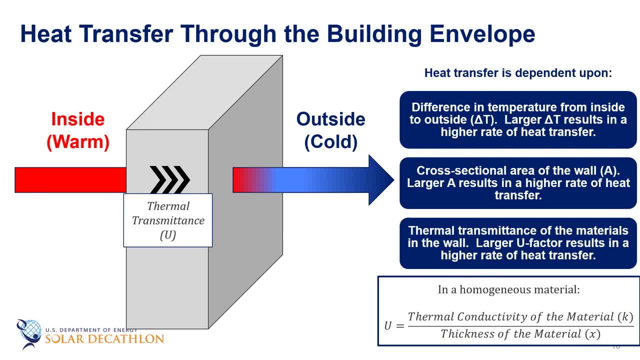 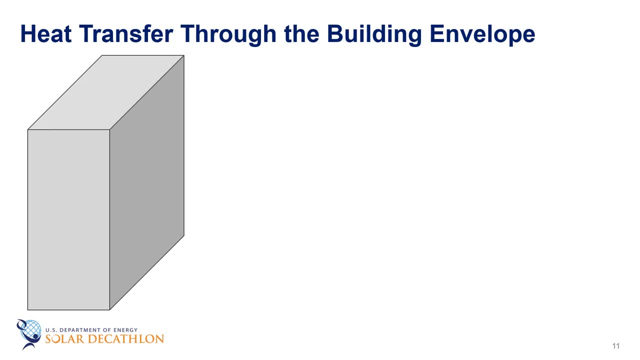 But we'll avoid going into more detail here. on thermal conductivity, If you'd like to learn more, this information can be found in any thermodynamics textbook or in the ASHRAE Handbook of Fundamentals. And so, coming back to our overview of heat transfer through the building envelope, 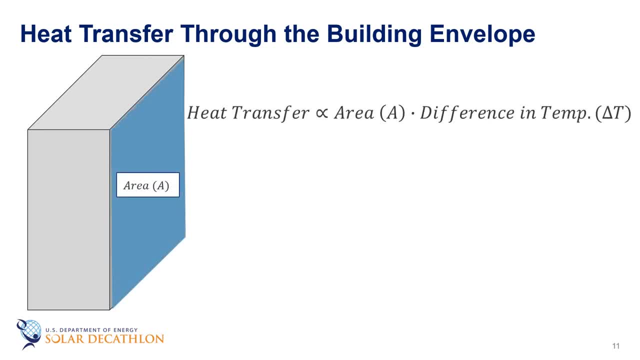 we talked about how heat transfer is proportional to the wall's cross-sectional area and the temperature difference from one side of the wall to the other, And we also discussed how we need a proportionality constant to bring these all together. The equation for the rate of heat transfer then. 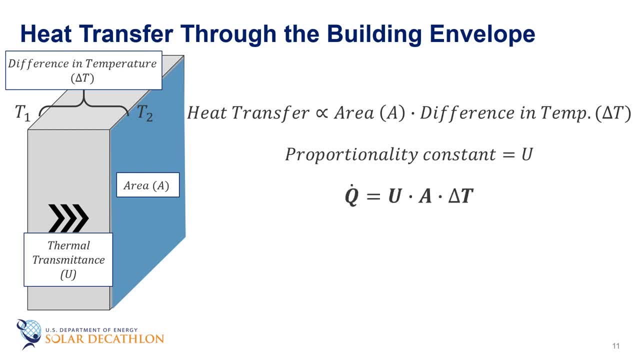 is Q. dot equals U times A times delta T. And if we look at the units for each of these terms, we can figure out the units of the U factor. I'll pause here to say that we're going to show units in the English system. 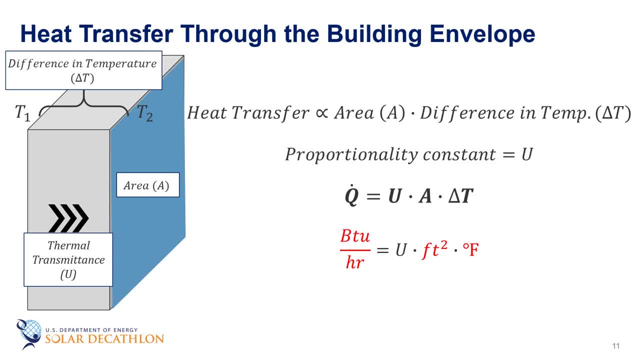 in order to be consistent with the building industry in the United States. However, other countries use the metric system. We'll provide a slide at the end of the episode with units for both English and metric for your reference. So, starting with Q, dot the rate of heat transfer. 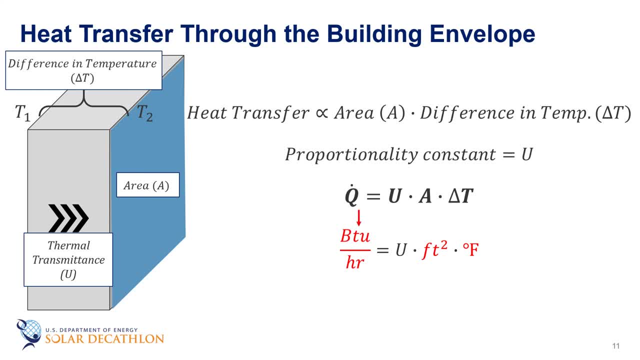 we know, those units need to be BTUs per hour. Area, then, is square feet, and delta T is in degrees Fahrenheit. That means that the units of U need to be BTUs per hour, square feet, degrees Fahrenheit, because the units of area and temperature will cancel out. 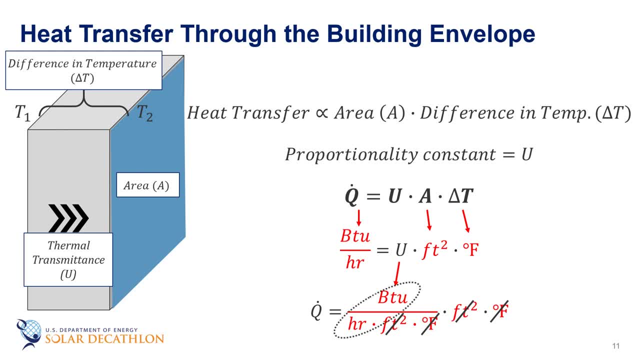 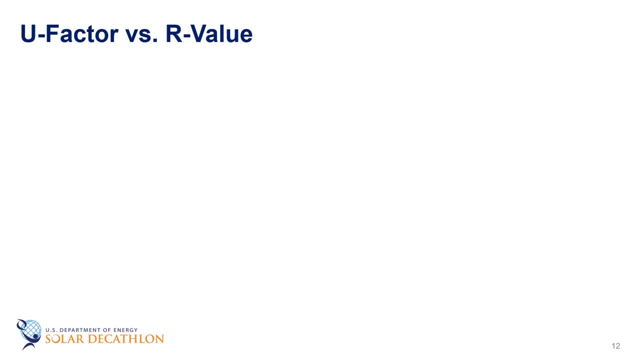 and leave us with our desired units for Q dot. Moving forward, we'll realize that there are two different terms used to describe how easily heat flows through a material: U factor and R value. The U factor, as we explained a moment ago, is the thermal transmittance. 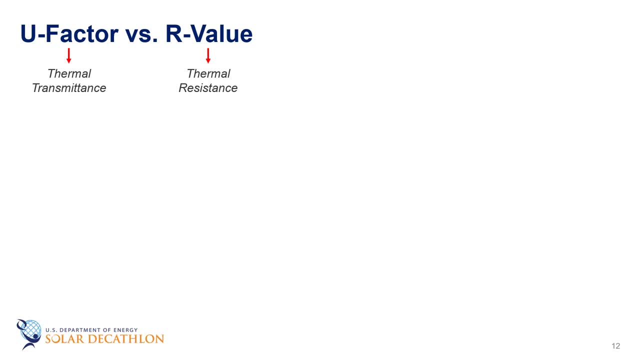 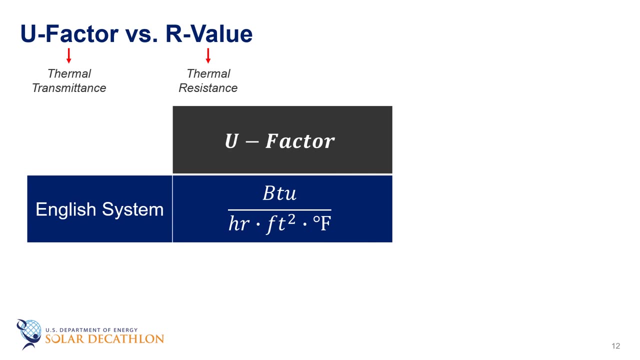 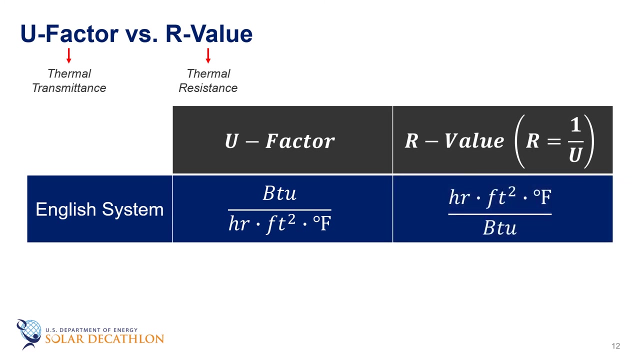 The inverse of this is the thermal resistance or the R value. So if the units for U are BTUs per hour, square feet, degrees Fahrenheit, and R is equal to one over U, then the units for R are hours square feet, degrees Fahrenheit per BTU. 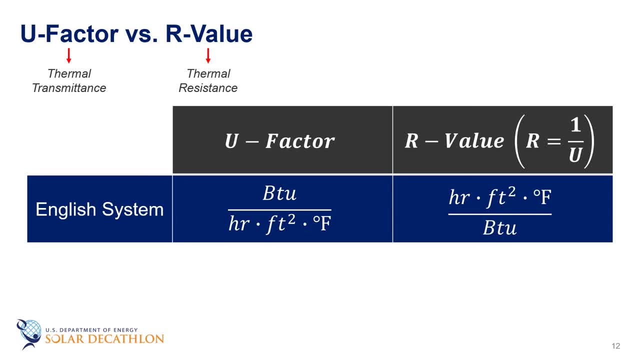 The higher the R value, the more resistance to heat flow. This R value is what you would most commonly see listed on the labeling for insulation products, and in the United States it's assumed that the R is measured in English units, as shown here. 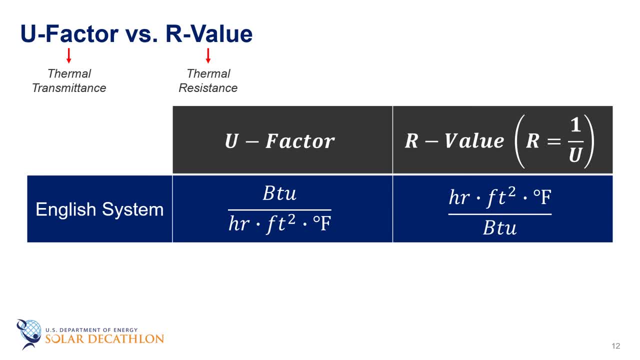 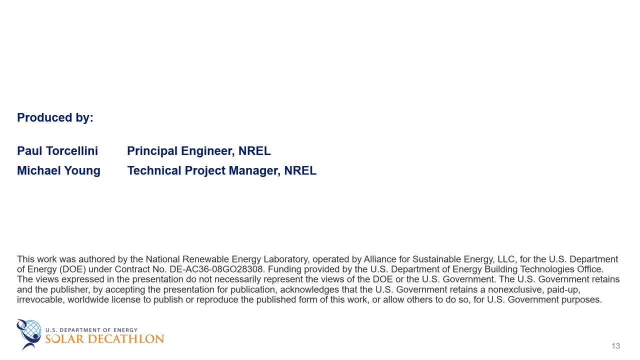 In other countries you may see this listed as RF, listed as RSI to indicate that the SI units are being used. We'll spend more time on R values in insulation in an upcoming episode And, as always, thanks for watching. 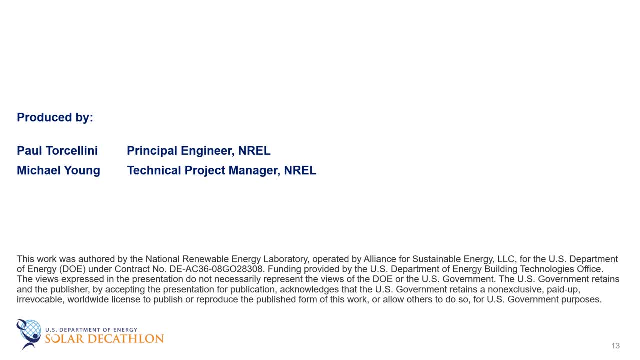 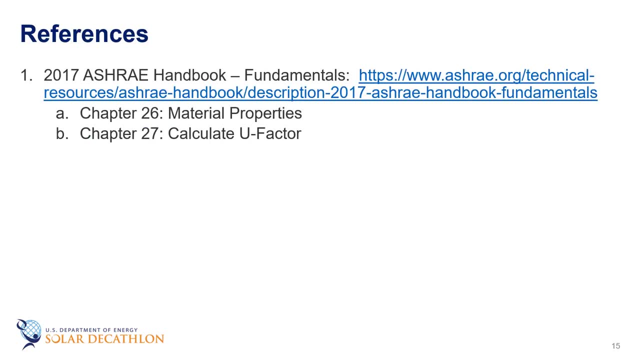 and please let us know if you have any questions or comments. See you next time.